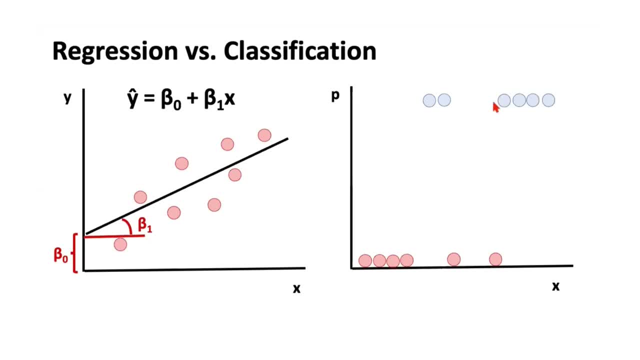 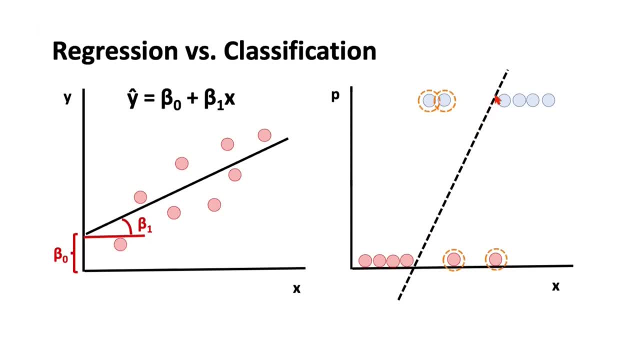 where we seem to be making errors, Because if we generalize with the help of this line, we would not make offers to these people, But in reality we know that these people actually went for a term deposit. Similarly, since these points are below the line we would have considered, 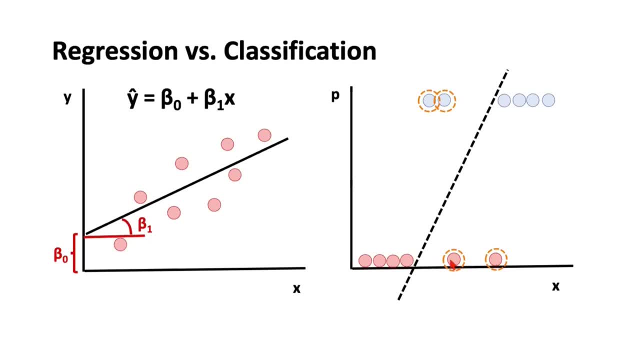 them for targeting, But that didn't be a mistake, because these people actually did not go for a term deposit. See, in supervised learning, the ground truth or the fact is already reported to us And using that fact and the historical data, we are trying to come up with a model. 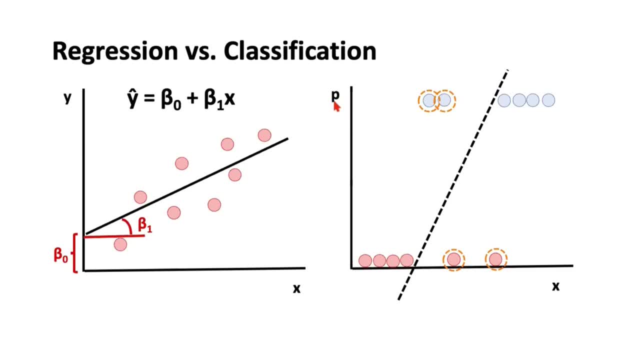 Notice that y-axis in this case represents a probability, because you are not predicting a value. You're predicting whether a given observation is likely to be a subscriber or a non-subscriber. So obviously we would not be able to do good with the help of this line. Notice in: 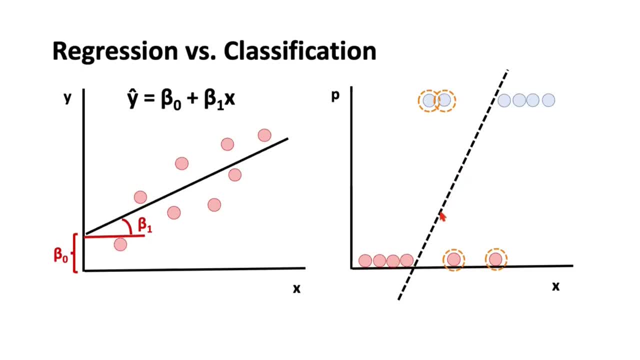 this case we are using a line not to represent these points but to segregate these points, And line may not be a batchwise as a segregator. but there are a couple of fundamental problems with the line. Let's understand those. So we've seen equation of simple linear. 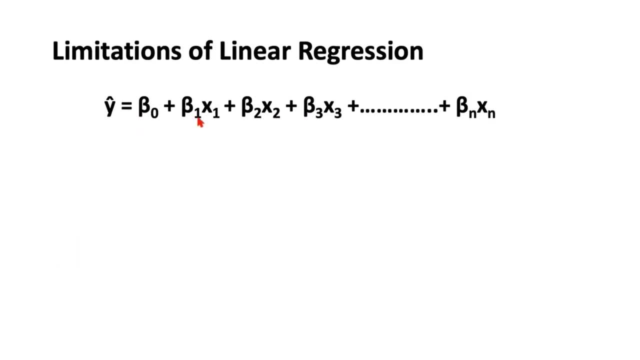 regression and multiple linear regression. The only change is that in case of multiple linear regression we add more variables and more coefficients. But there are two main issues. if we are using a line to predict the probability, What are those? Number one: probability always lies. 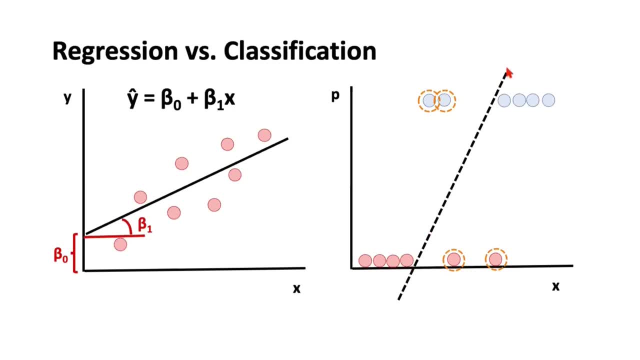 between 0 and 1.. So, if you see, in this case this line may not necessarily be restricted to 0 and 1. only A line can extend from negative infinity to positive infinity in terms of y value. How are we going to ensure that this is always between 0 and 1?? 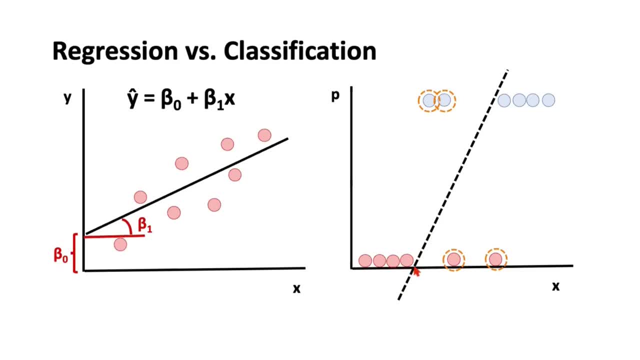 Let's say that we'll probably do some kind of a camping at 0 and 1 and say that if it's below 0, we'll bring it to 0. If it's above 1,, then we'll bring it to 1.. So you can put some restrictions. 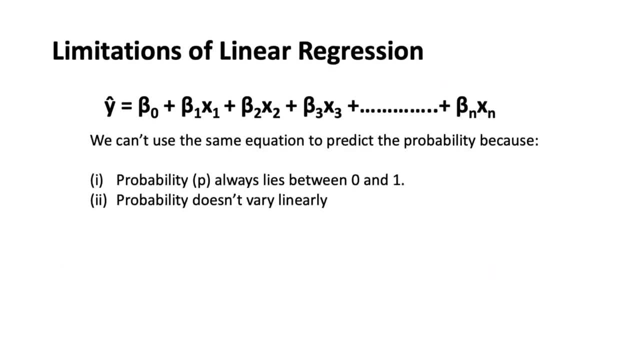 on that. Then comes the second problem. And the second problem is bigger. The probabilities don't vary linearly. What does it mean? Let's understand this with the help of an example. So let's say we are talking about achieving 10% score improvement in the exams. Now event A is when your current 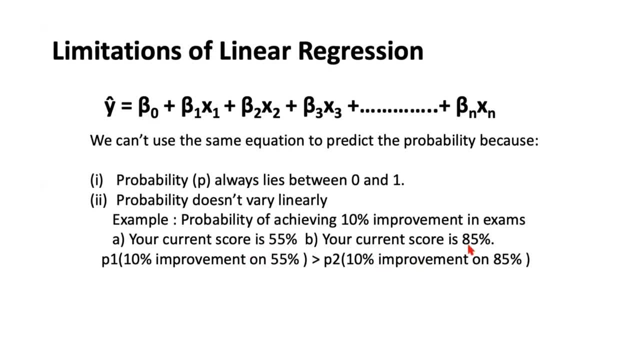 score is 55% And event B is when your current score is 85%. A is represented by the probability P1. And event B is represented by the probability P2.. Without much deliberation, you'll be able to think that most likely P1 will be greater than P2.. 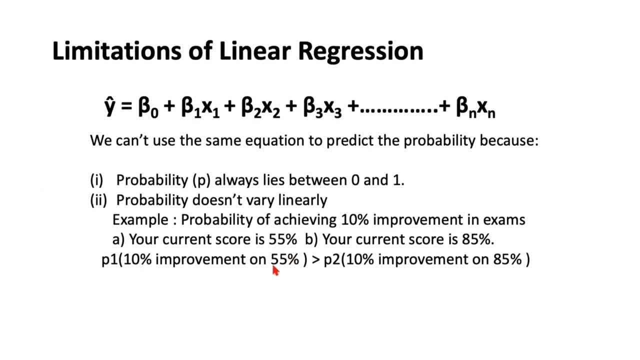 Why? Because if you're at 55% score, there is a larger room for improvement. Achieving another 10% improvement is going to be easier. You're talking about the same exam, Whereas a person sitting at 85 hardly has any room because your score can't be above 100%. 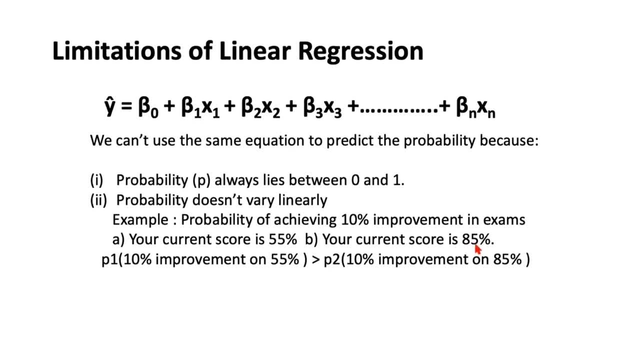 So this person might have already tried his best To be able to achieve 85%. any further improvement would require a lot more effort, a lot more command on the subject, Whereas for this person the hopes could be high, because in the same exam somebody is already achieving 85%, Whereas this person is at 55. So there's a 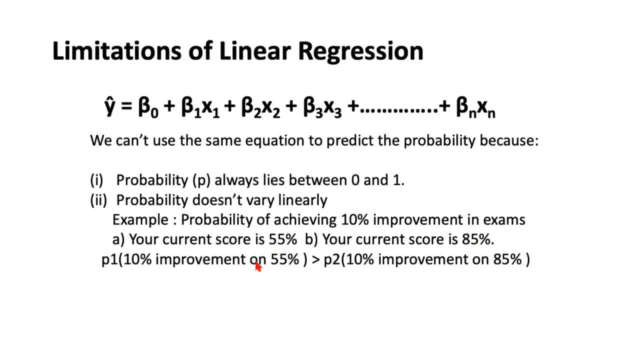 high chance that this person can improve. Again, we are talking in terms of probability, But the idea was that probabilities don't vary linearly, So how justified would it be to make decisions related to probabilities based on a line, Which means we actually need a link? 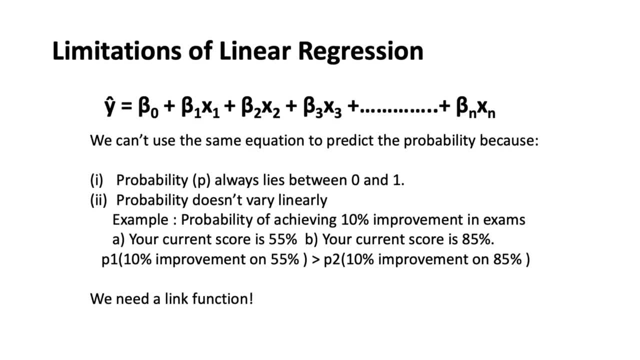 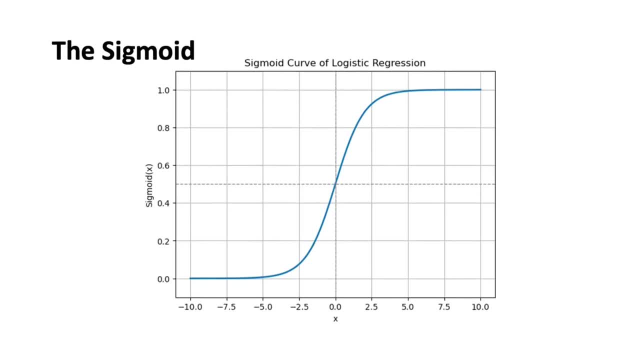 A kind of function which is not a line and it is always confined between 0 and 1. And the answer to this comes in the form of the sigmoid function. So in calculus, if you've studied different functions, you would know that a sigmoid function is a function which 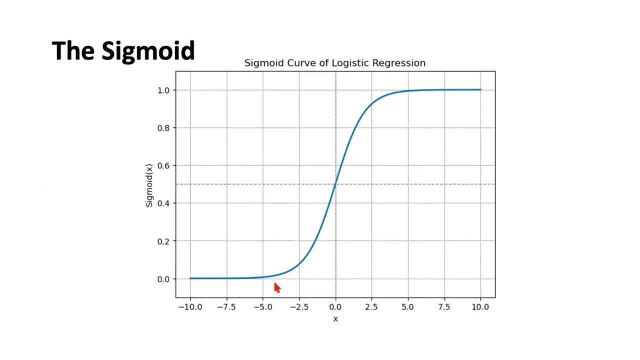 always lies between 0 and 1,, no matter what the value of x is, And it is, of course, nonlinear. How would it act as a classifier for us? Let's understand that. So imagine this is the kind of decision that we have to make, right? So we have these points. which are the people not to be. 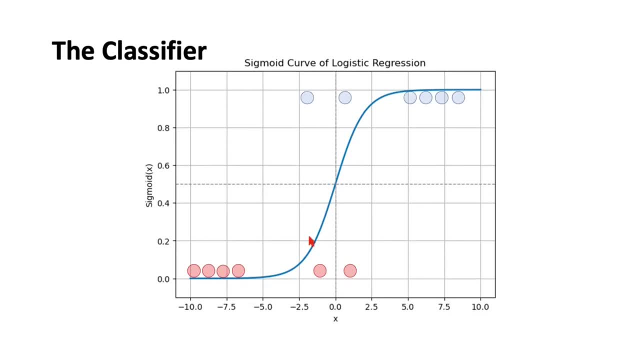 targeted. And we have these points which are the people not to be targeted, And we have these points which are the people not to be targeted, And we have these points which are the people We are able to draw this kind of a curve which doesn't vary linearly. Notice that you might. 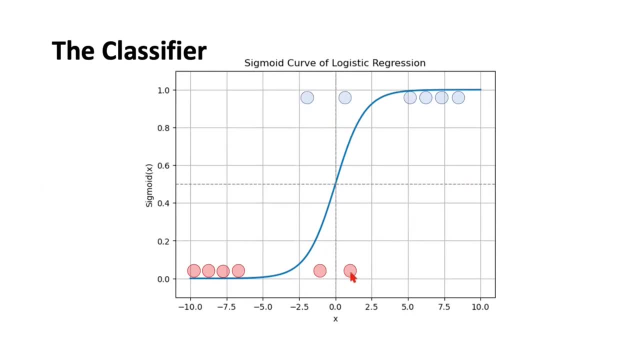 still say that this curve also seems to be making errors, which is fine, but at least it is not violating the fundamental assumption. It is still operating in the range of 0 to 1, which is very much like probabilities, and it is nonlinear. Now can we fine-tune this curve to ensure that? 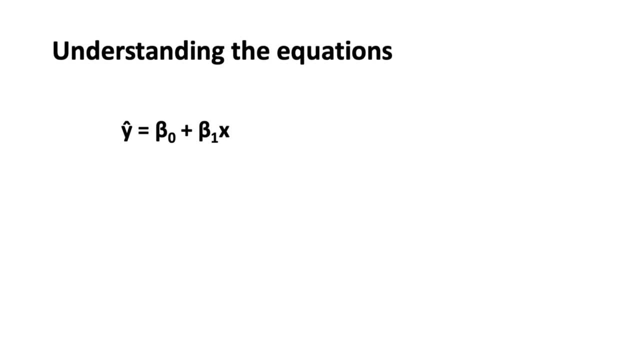 we reduce the error. Let us understand, in terms of expressions or equations, how does logistic regression look like. So in case of linear regression, we are able to draw this kind of linear regression. We know, in simple, one-variable scenario we had this equation: Y hat is equal to. 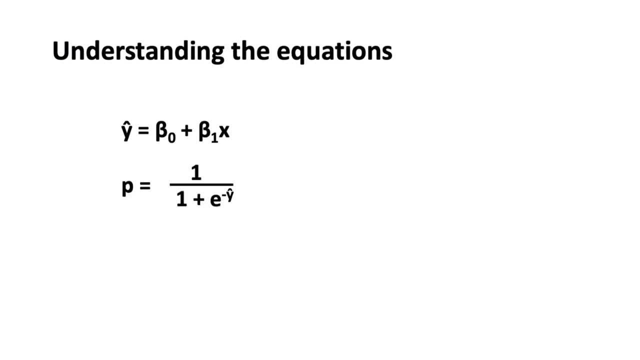 beta naught plus beta 1 x. In case of logistic regression, we are predicting probabilities and we are using the sigmoid function. So the equation is like this: Probability is equal to 1 over 1 plus e, which is a constant raised to the power negative y hat, where this y hat is still. 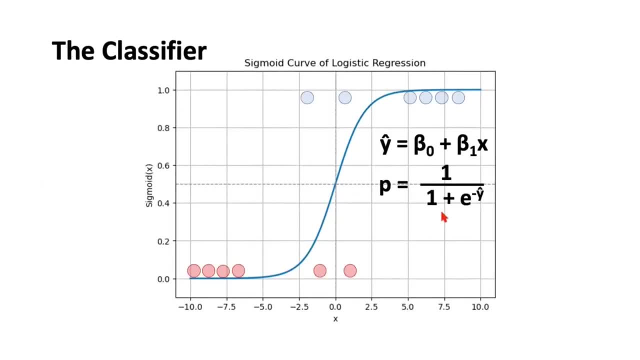 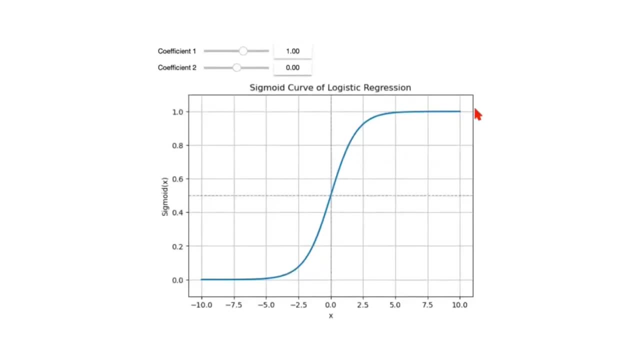 equal to beta naught plus beta 1 x. So let's understand what will be the influence of beta naught and beta 1 on the probability of this regression. So let's understand what will be the influence of this regression. So here we are. We have the same sigmoid function and we have 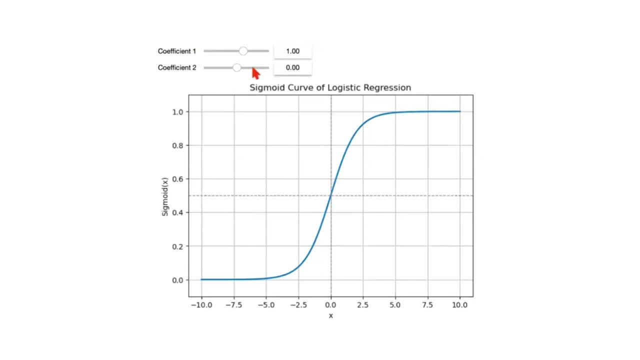 the coefficient values which we can adjust right. So let's just see if we take this coefficient 2, which is in this case beta naught- If we take this to a little lower value, what would happen. You see, the shape of the sigmoid is kind of changing, And if this is how the shape of the 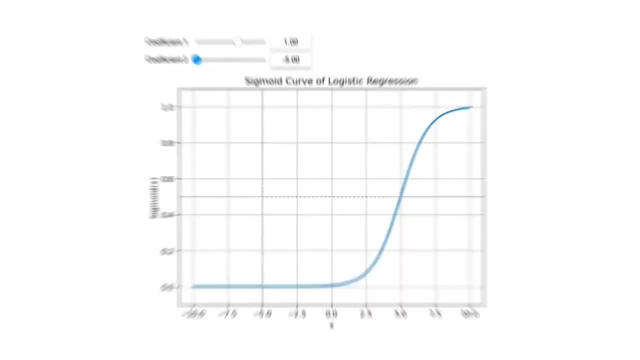 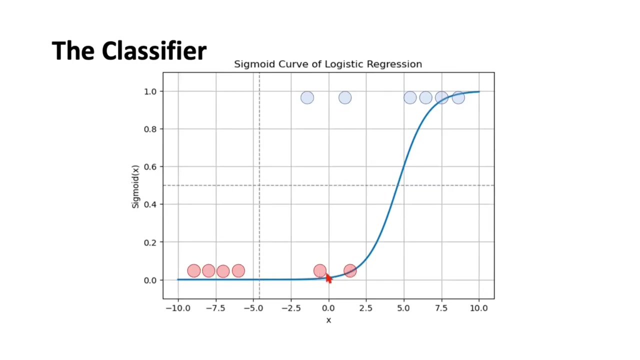 sigmoid is. what would it mean to our classification problem? Can you imagine we are looking at a scenario like this? So earlier these two points were the same, but now they are different. So these two points were misclassified. But now these two points are being properly classified. 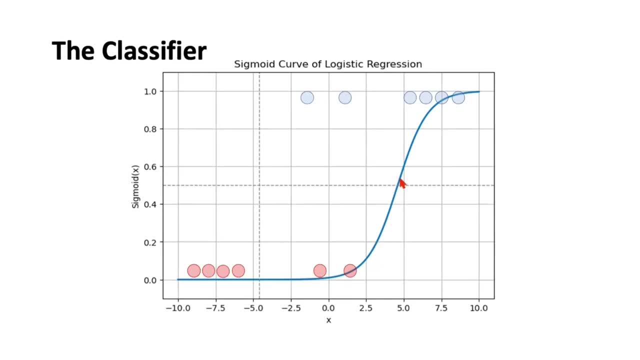 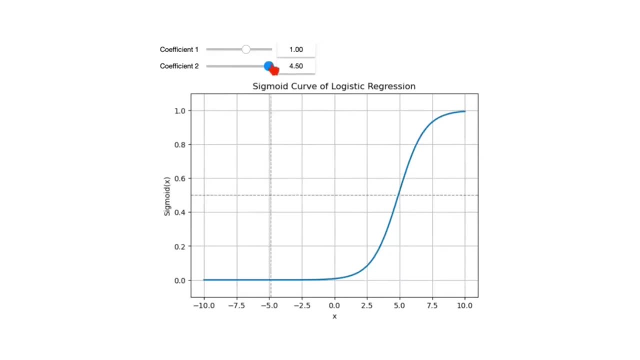 because they are being covered as the sigmoid function on one side. Likewise, if we increase the value of this coefficient 2, then what happens? Let's say, we bring it to this extreme, Then what happens? Do you see, the shape of the sigmoid function is kind of changing. 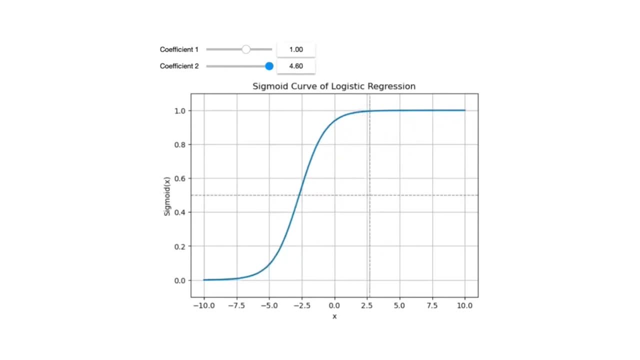 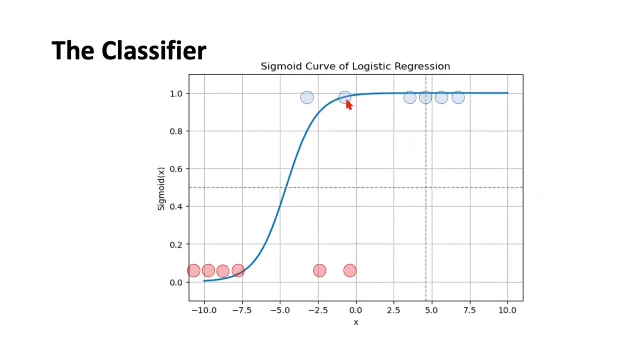 Still a basic n-shaped curve, but you can see it is changing. And now what does it mean to our classification problem? It is something like this: So this point, which was earlier being misclassified, would be classified properly. Notice, we still would have some. 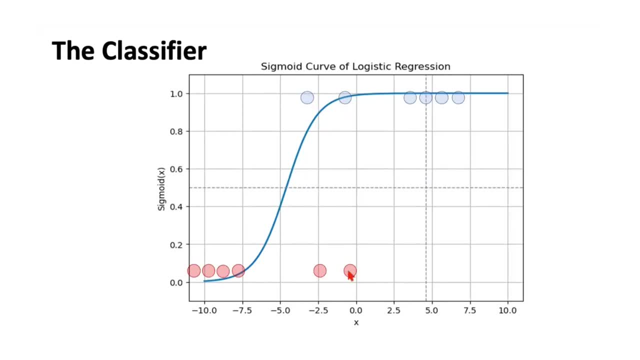 errors. For example, this remains an error and these two points also remain errors, But changing the values of the coefficients would make a difference to the sigmoid function and we'll accordingly be able to tune our model. This is what we did in case of a line We could draw. 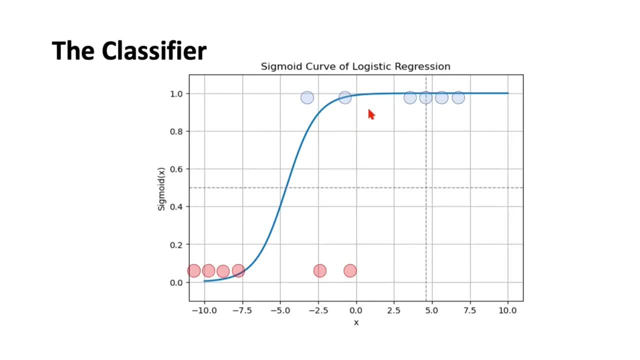 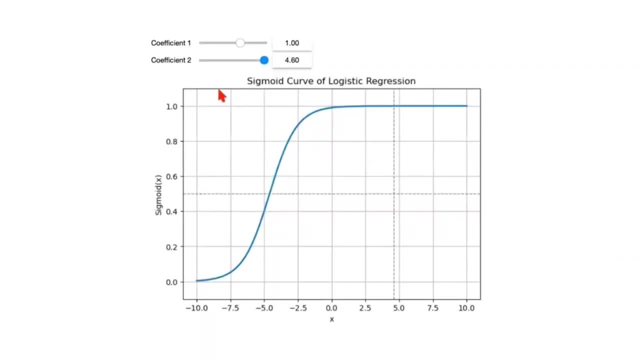 multiple lines, but we settled for the line with the least error. And how did the line change? The line changed by adjusting its coefficient. Here the sigmoid is changing by adjusting the coefficients. So I've only changed the values of constant, which is beta naught. We adjust the coefficient. 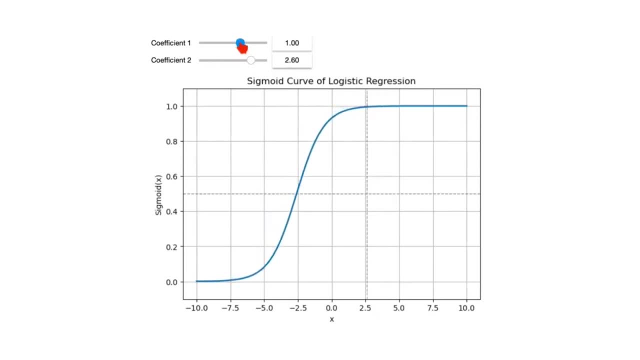 somewhere in between and also try to change the values of the coefficient beta 1.. And let's see what happens. Do you see Sigmoid entirely changed? If I move it here, then what happens? So this is a nice visual representation. How does a sigmoid curve get affected when you change the? 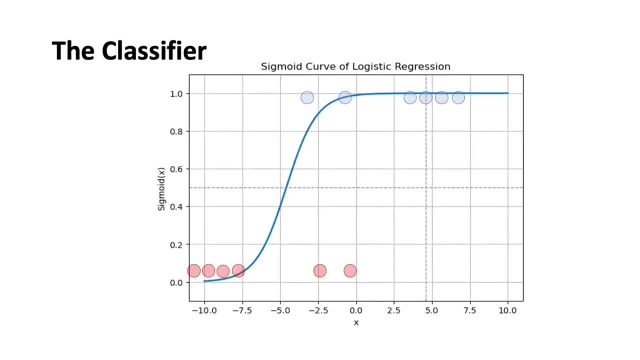 coefficient values. Hope you get the idea. You may be wondering: in case of linear regression, we had a simple linear regression which had just one independent variable. We've seen one independent variable which had just one independent variable. So we have a simple linear regression. 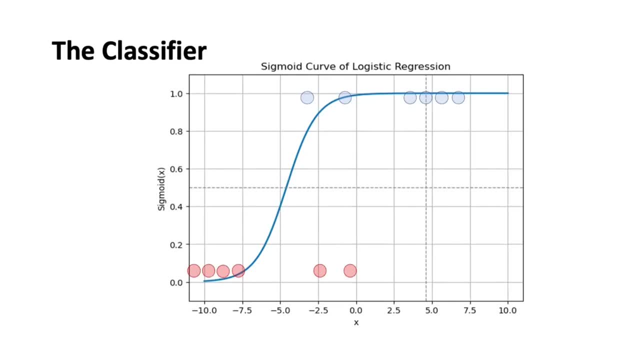 and how does it affect the logistic regression? But in regression we also studied multiple linear regression, which means when you had more than one independent variable. how does it affect the outcome, What it would be like in case of a logistic regression? So this is another visual. 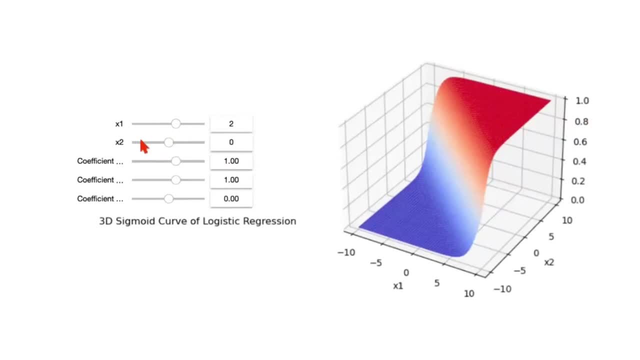 representation. Let's say we have taken another variable to explain the outcome. Instead of just one variable x, we have a variable x1 and a variable x2.. These two variables are trying to explain an outcome. Now, instead of just one coefficient, we will now have three coefficients. There is 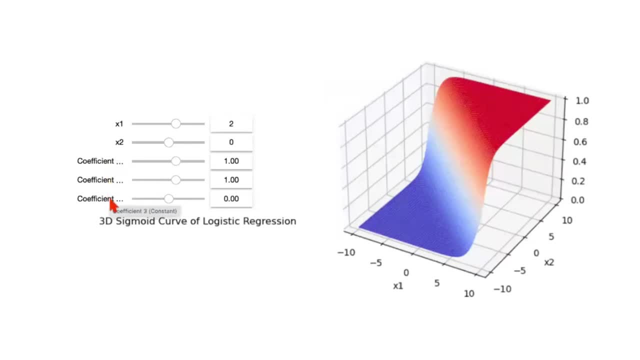 coefficient 1 for x1,, there is coefficient 2 for x2, and then there is a constant term And there are some default values. But why I brought you here is because I wanted to show you how does it appear in a multidimensional space. So you can imagine. this is like a paper, which is kind of 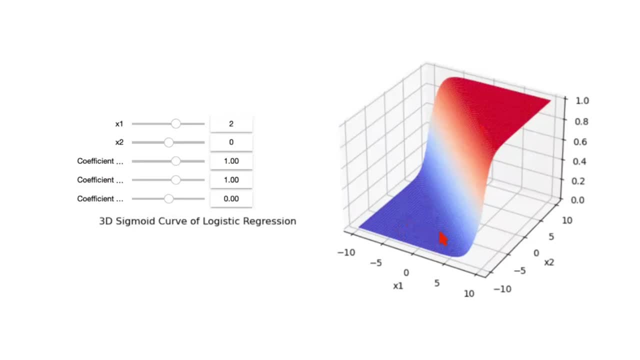 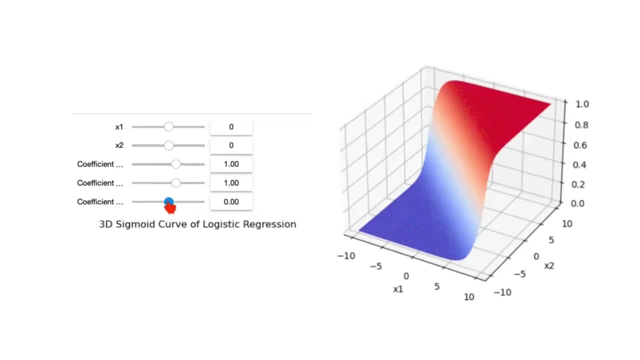 a little rolled paper which you're trying to open. So it is again forming an S kind of a shape And in the multidimensional space it's called a hyperplane. right, We can try to change the values of the coefficients and the constants and see how does it affect the outcome. Let's say I'm 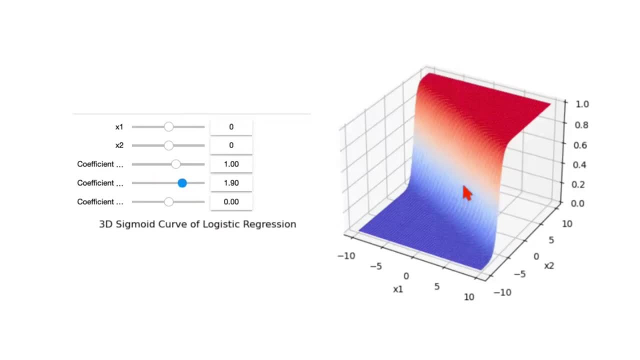 trying to change one of the variables. Do you see? its shape is further changing. The paper is kind of rotating. And let's say we try to change this variable as well, then what happens? It's going in the other direction. So if I reduce this further, what would happen? You can see this. 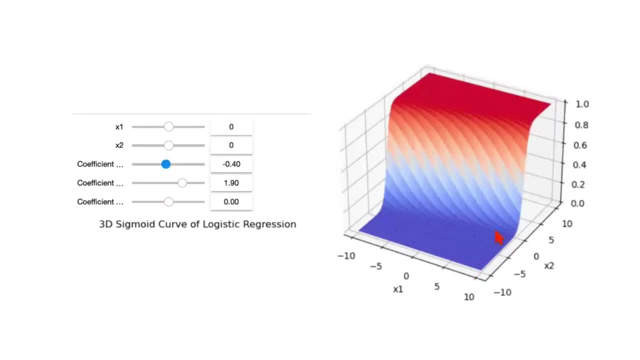 is how it's. it's clearly looking like an S shape. If you look at it from one side, let's say from this direction x2, sideways- it will exactly look like a sigmoid function to you, right? So I hope you get a better idea that what we saw in a 2D would be translated into 3D. Unfortunately, we will. 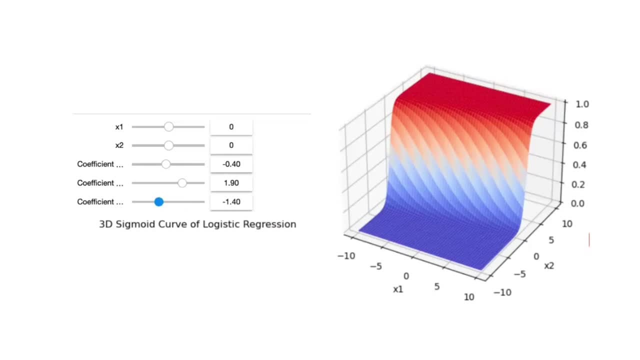 have to demonstrate more than three dimensions, typically through this kind of visualization, So we limit it but hope you get a clear understanding that what a sigmoid is like and how is it interacting. What are these axes? This is our first independent variable. This is our second. 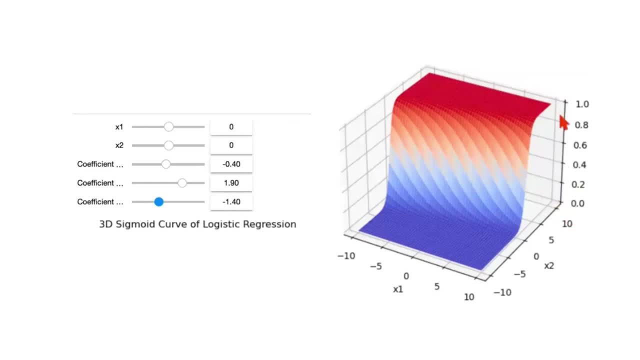 independent variable, And this is the probability that we are predicting in a range of zero to one. So no matter what stays between zero and one and can accept values for the independent variables, These were just some dummy values that we started with on a scale of negative 10 to 10, just to. 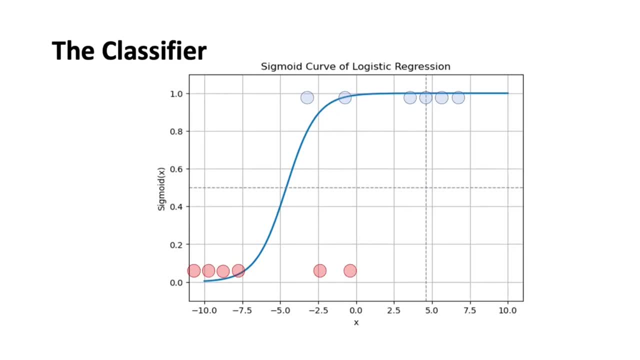 visually demonstrate it. So we understand that changing the values of beta one, beta, two, beta not affects the sigmoid function. But how do we settle for the right values for these coefficients? That's what we're going to understand next For our example. right now let's just consider only six points. Let's 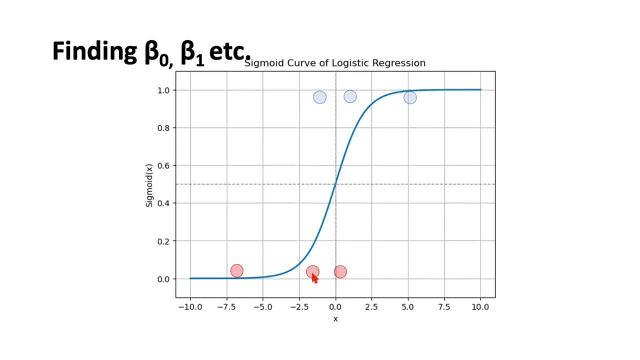 say we have these three points, and these three points, These three points here represent the event where we don't want to target the prospects, And these three points represent the event when we want to target the prospect, We want to pitch the term deposit to these people and we don't want to. 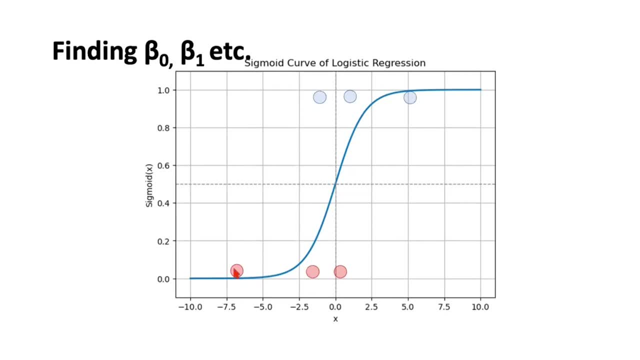 target these people. So what should be the case? How should the probabilities be looked at? One is: this is an ideal case where this probability is almost close to zero. When the probability is almost close to zero, you're saying that you're not going to target this prospect. You're not. 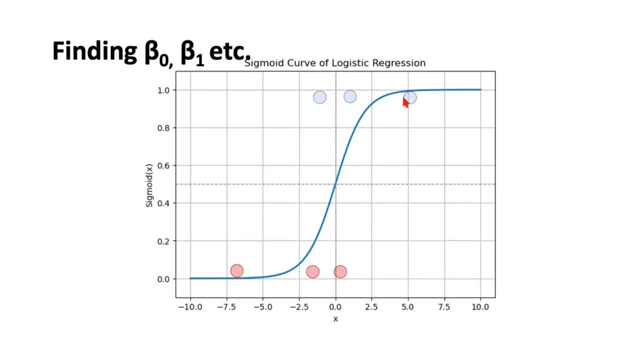 going to pitch This case is also very clear when you're saying the probability is almost close to one, which means you're definitely going to pitch the term deposit to this. But these points here are somewhere in between and, in fact, misclassification. In fact, that's the very 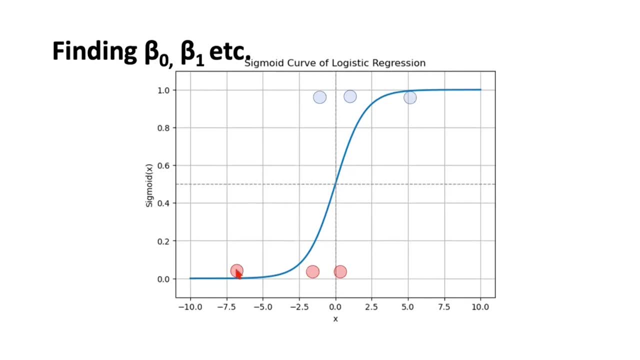 reason that we kept these here as examples. What is the probability corresponding to this point? Almost zero. What is the probability corresponding to this point? Almost one. What about the probability of this point, this point, this point and this point? This will be obtained by taking: 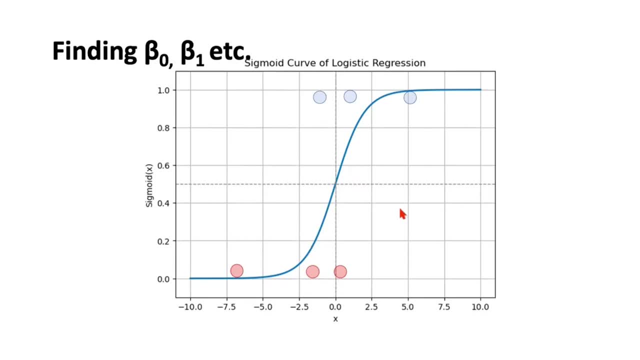 the corresponding value on this sigmoid curve. So if I were to show you a little clearly, P1 is almost zero, P6 is almost one, but all the other probabilities. for this second point, probability is this point on the curve. For this point, this is P4.. For this point, it is P3.. For this point: 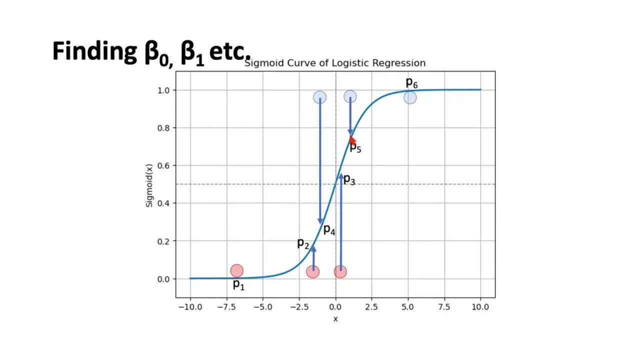 it is P5.. These are the corresponding values on the sigmoid curve. Note that we want P1, P2 and P3, the probabilities corresponding to these red points- to be as small as possible And we want the probabilities corresponding to these blue points- These are P4, P5 and P6- to be as high as possible. When I say as high, the max is. 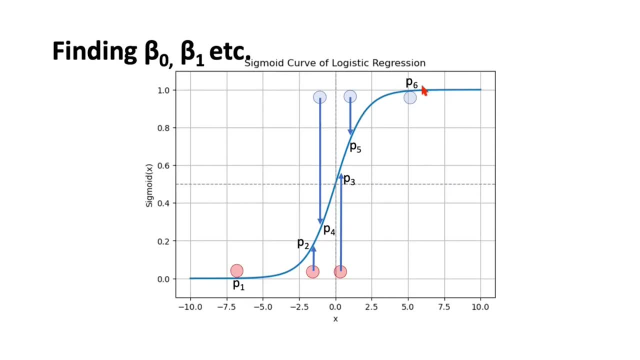 one to as close to one as possible. There is a slight conflict. For some points, we want the probabilities to be minimized. For some points, we want the probabilities to be maximized. What if we are able to write this in such a way that, for all the points, the probabilities are to? 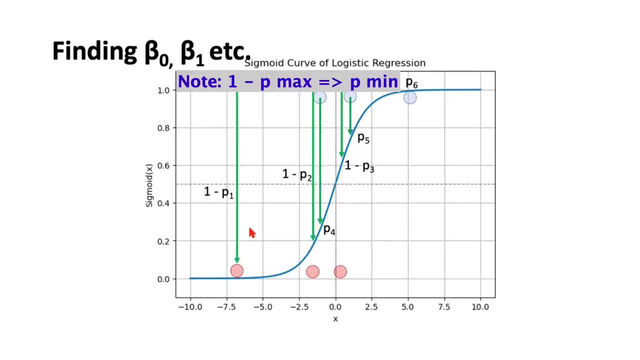 be maximized. Can we do that? Actually, there is a way out, And it's like this: Instead of writing as P1, if we write one minus P1. So if we say one minus P1 is to be maximized, that implies P1 is. 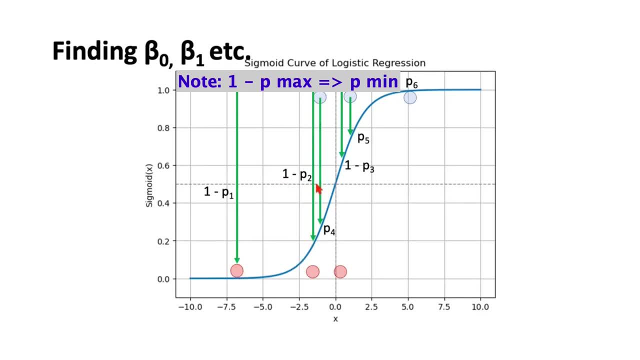 to be minimized. Similarly, if we say one minus P2 is to be maximized, P2 will be minimized As such. P4, P5 and P6, we don't have a problem with. We always wanted them to be maximized. 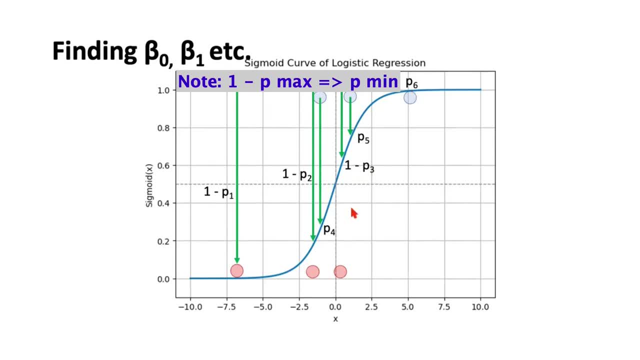 Because we wanted them to be close to one. And again for P3, if P3 is to be minimized, then one minus P3 is to be maximized. So we have written all these probabilities in the terms where we are talking about them in one direction and their maximization. So remember: 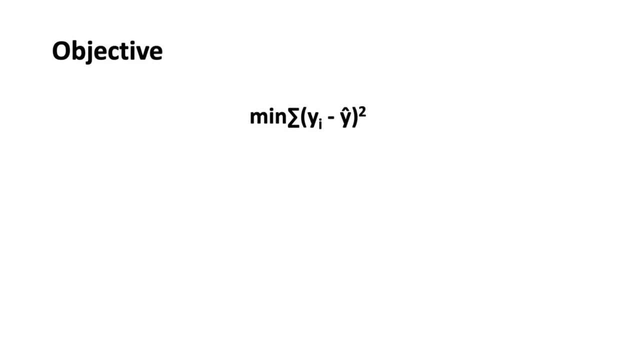 any machine learning problem would always be solved keeping an objective in mind. In case of linear regression, we had this objective. The squared differences between the actual and predicted values added up is something that we wanted to be minimized. Sum of a squared factor. What is this objective in case of logistic regression? In case of logistic regression, this is: 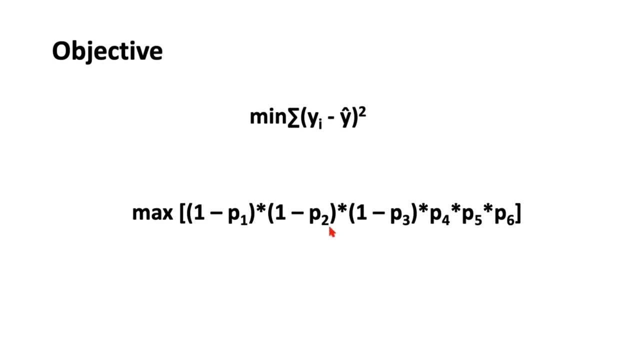 the objective The same thing that we just discussed: The one minus P1, one minus P2, one minus P3, multiplied by P4, P5 and P6.. All these asterisks represent products, So all these products taken out should be maximized. We are looking for such values of coefficients which 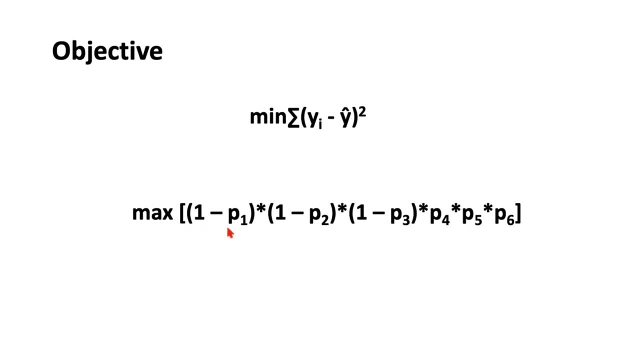 give us the maximized output for this equation. Now imagine we have just taken six points. It could be multiple points, But the fundamentals stay the same. This is known as the maximum likelihood. You might have heard about this term if you've dealt with statistics. Now one word of caution: Maximum likelihood is: 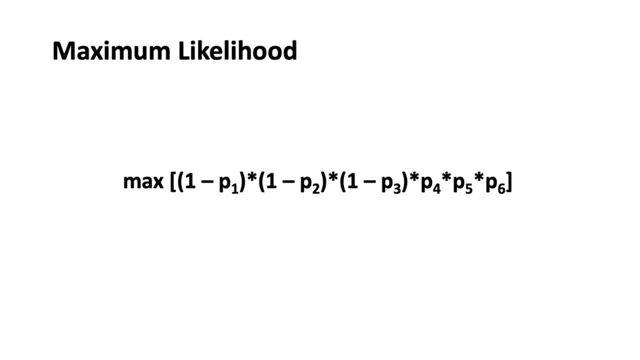 not the same as probabilities In terms of common interaction. in English we use probability and likelihood interchangeably, But likelihood is ideally a term you want to use when you're trying to estimate something using probabilities. So we are using the probabilities here and we are 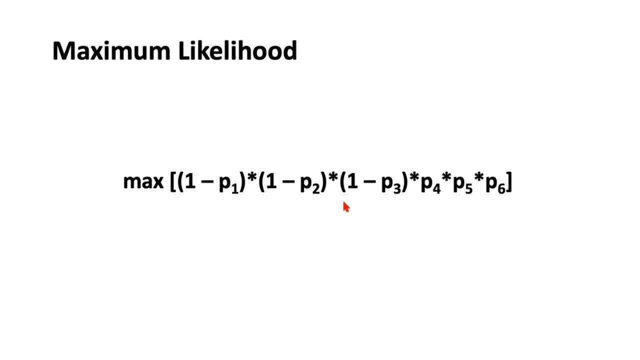 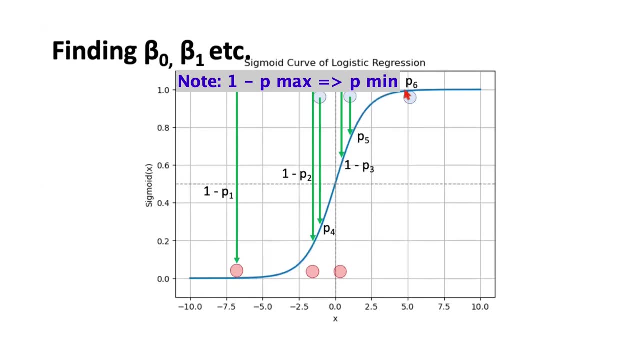 trying to estimate what, Not the probabilities, but the coefficient. That's where likelihood plays a role. Alright, So with this, so far we've already covered that sigmoid is the solution because it stays between zero and one, It is nonlinear, And we also learned: 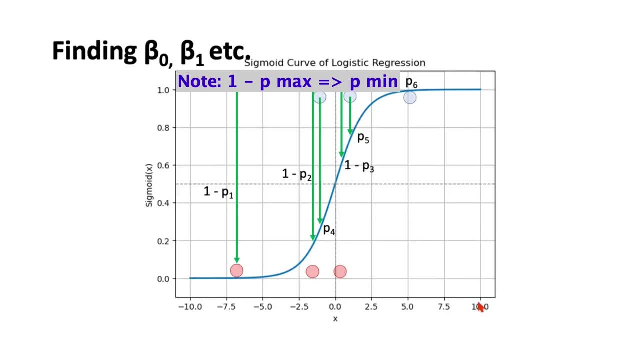 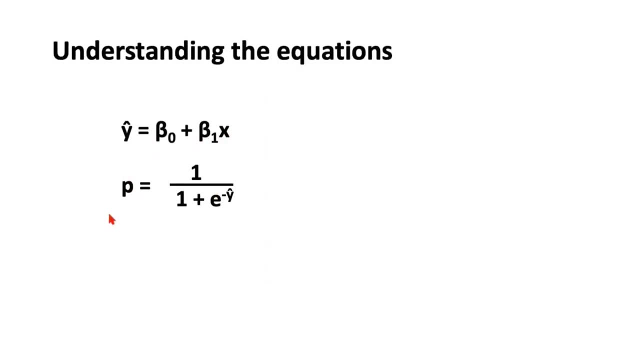 about the objective. Let's understand a little bit about the kind of expressions involved in case of logistic regression. So we've already seen these expressions. This is a simple linear regression. This is the equation to derive the probabilities using the sigmoid function. y hat here is the same as beta naught plus beta 1 x. 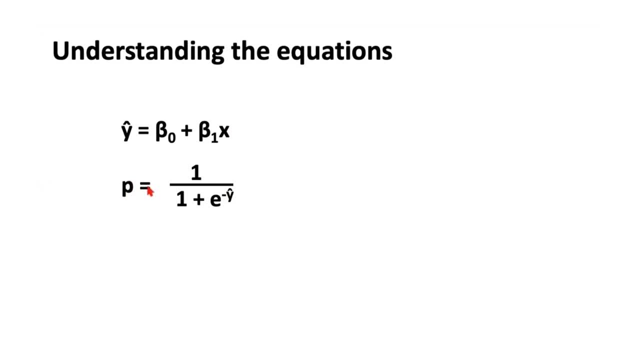 We have, can we do slight changes and we are aware of how to get the probability using y hat, But is there a way that we can get to know how we can get y hat using probabilities? What I mean to say is this: Can we do some manipulations to this expression? Let's say we do one minus p, If you. 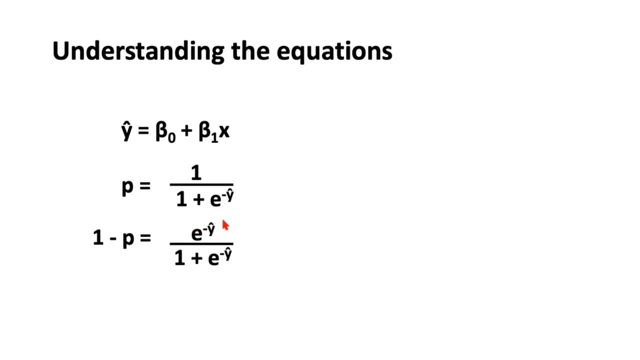 try to do this on your own, you will realize that the right hand side of this expression then would be this: And what if we divide the first expression by the second expression? We divide this by this. What we're going to get is something like this: You may try that on your own. 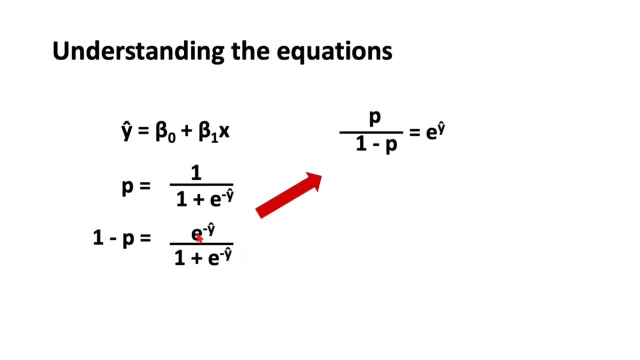 If you do this, the denominators would get canceled. You will have 1 over e raised to the power negative y hat And that can easily be written as e to the power of y hat. Now we're just one step away in getting y hat in terms of probability, So we'll have to take the log to the 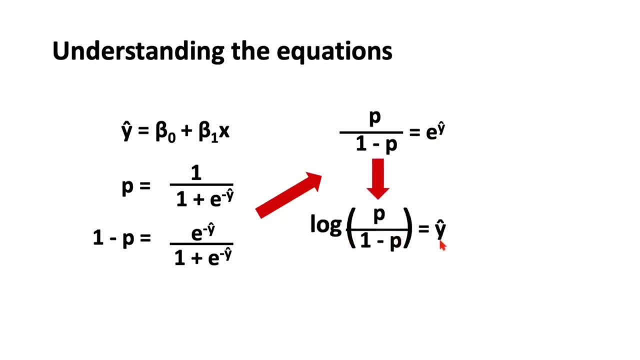 base e on both the sides, And what we get is this: So y hat is log of p over 1 minus p. By the way, what is this p over 1 minus p? This p is the probability of occurrence of the event that we 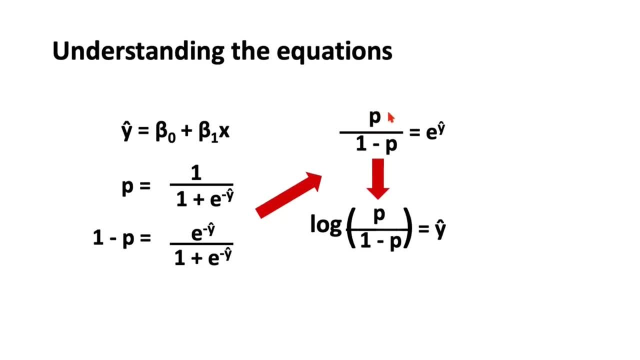 are interested in. In our example, this was the event of a prospect agreeing for a term deposit And 1 minus p in that case would be the prospect not agreeing for a term deposit. This is a case where we should have targeted because the prospect is likely to agree. This is the case where we should have not targeted. 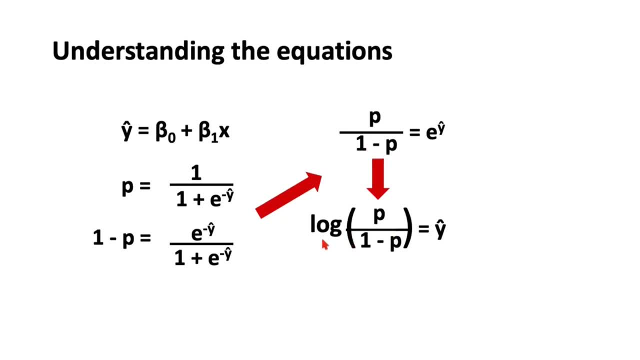 the prospect, because prospect is less likely to agree, And this is called the log odds ratio. So what is this? y hat? Once again, using this expression, we can say: this is beta naught plus beta one x. So in case of logistic regression, 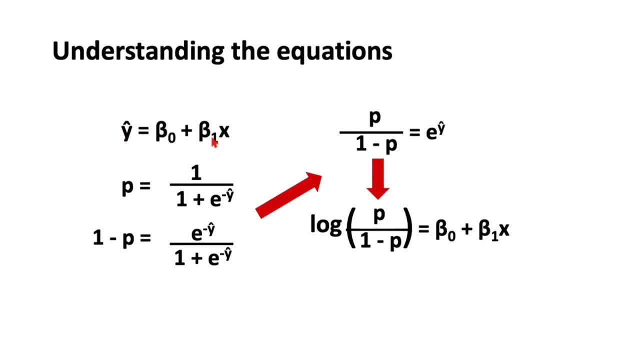 you don't have a linear relationship between y, hat and x. That was the case with linear regression. In case of logistic regression, you have a linear relationship between the log odds ratio and x. This is actually one of the assumptions for logistic regression. And what would happen if we? 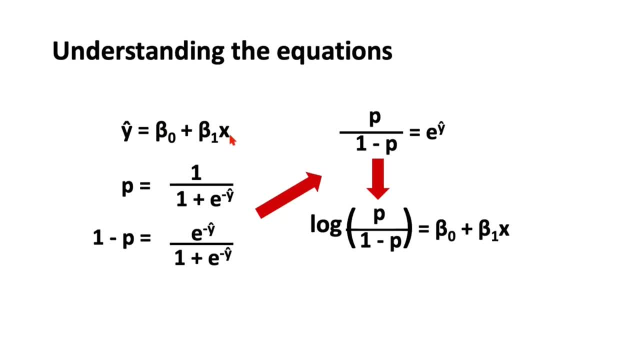 have one more variable Instead of just x. let's say we have x one and x two here. If that's the case, then you will expand your expression. Instead of just writing beta one x, you will write beta one x one plus beta two x two. And similarly for the log odds ratio, you will write: 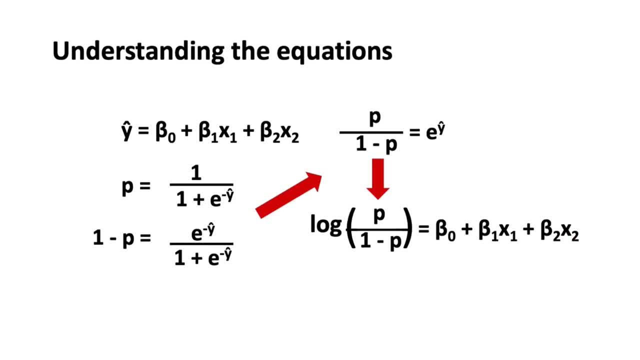 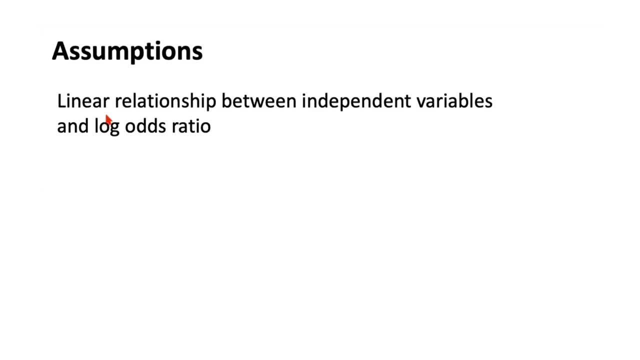 beta one x one plus beta two x two. So that's about the basic expressions. Let's quickly understand the assumptions involved in logistic regression. Some of these are common, as we saw in linear regression. So the first one is: we've just now discussed that there has to be a linear 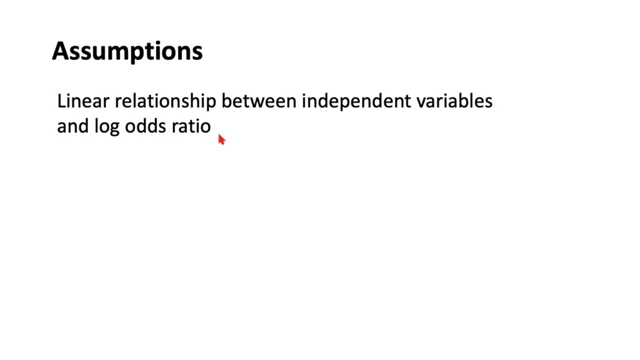 relationship between the independent variables and log odds ratio, log p over one minus p. This is a common assumption of multi-collinearity that we had with linear regression as well, that we do not want independent variables to be relative. So when you have more than one variable involved, let's say x one, x two, x three, you do not want. 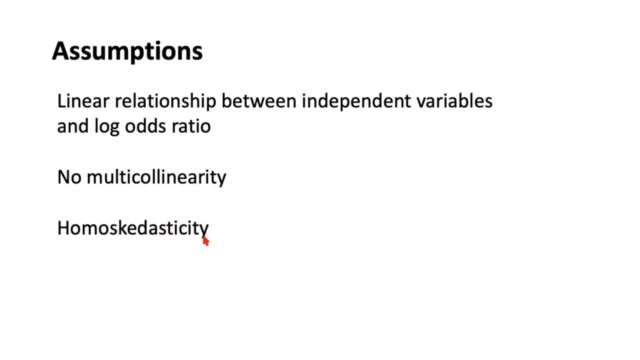 variables to be correlated to each other. We also discussed something called as homoscedasticity, which was about the constant variance of the error terms That stays the same. Notice that logistic regression does not have any assumption about the normal distribution of the errors, but it